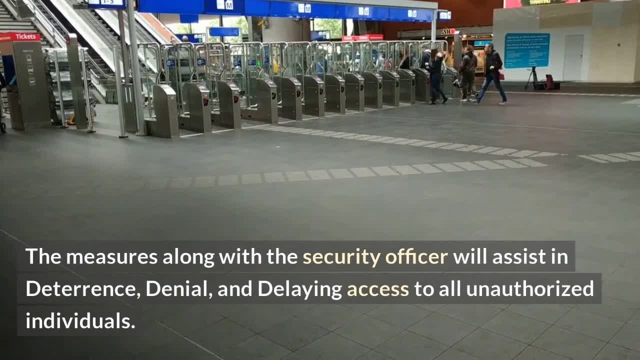 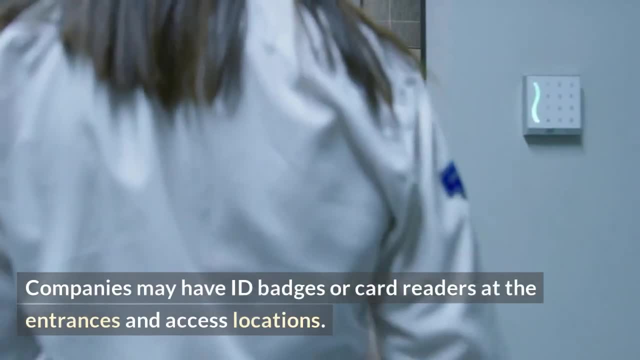 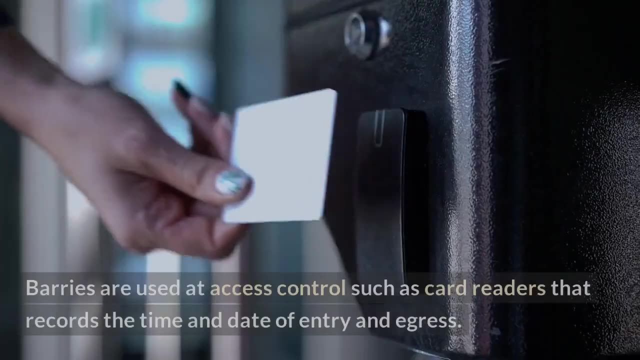 infrastructures. The measures, along with the security officer, will assist in deterrence, denial and delaying access to all unauthorized individuals. Companies may have ID badges or card readers at the entrances and access locations. Barriers are used at access controls such as card. 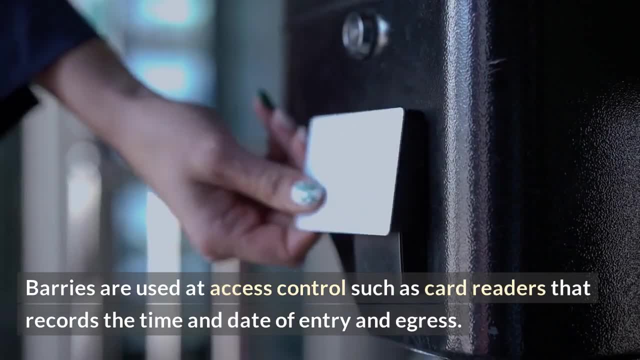 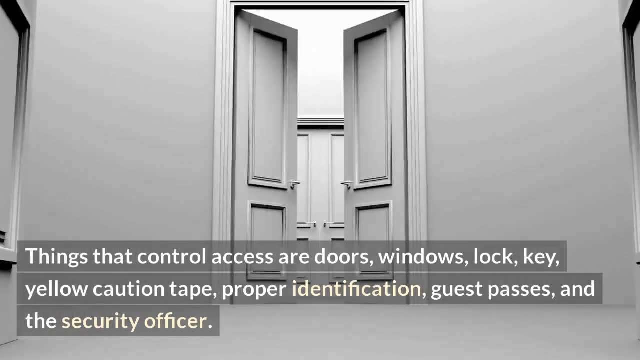 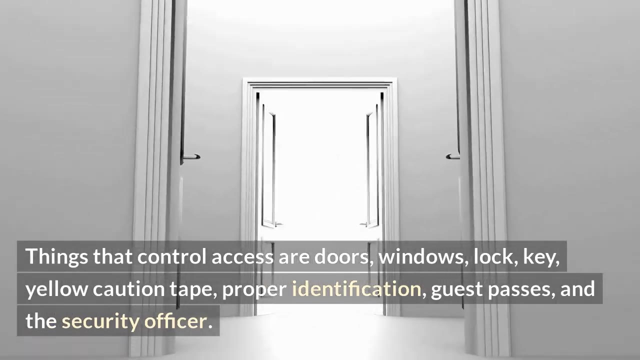 readers that records the time and date of entry and egress. These barriers include turnstiles or card swipes. Things that control access are doors, windows lock, key, yellow caution tape, proper identification, guest passes and the security officer. During your patrols, you will physically 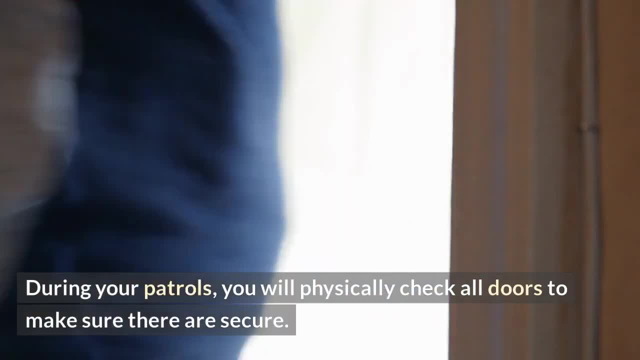 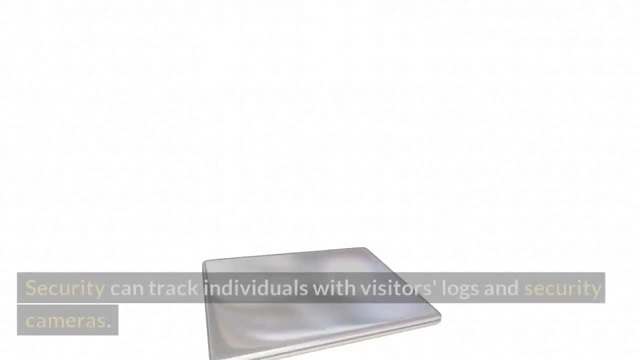 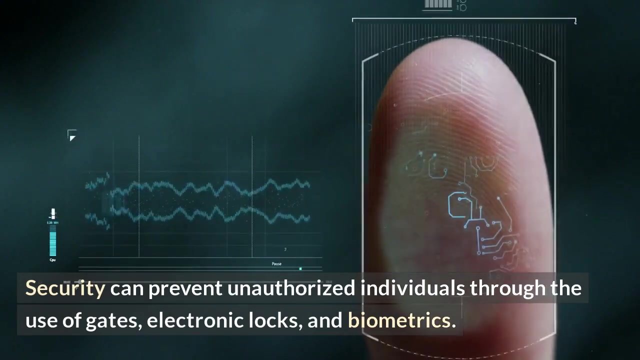 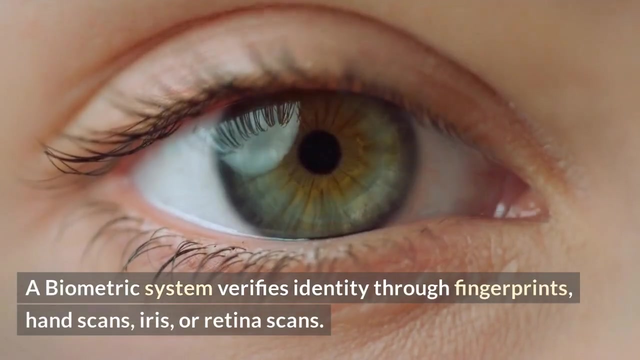 check all doors to make sure they are secure. Access control can track entrances and exits. Security can track individuals with visitors' logs and security cameras. Security can prevent unauthorized individuals through the use of gates, electronic locks and biometrics. A biometric system verifies identity through fingerprints, hand scans. 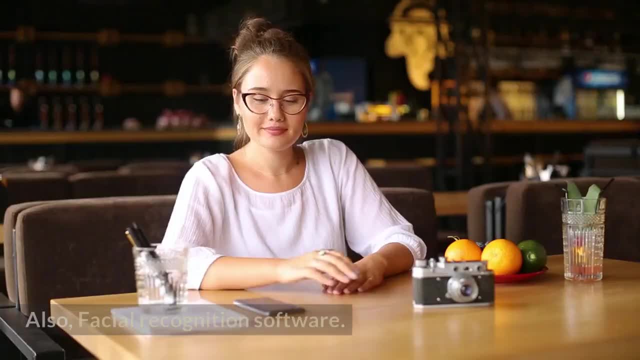 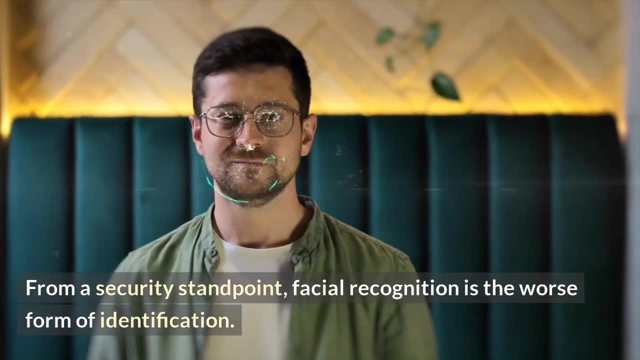 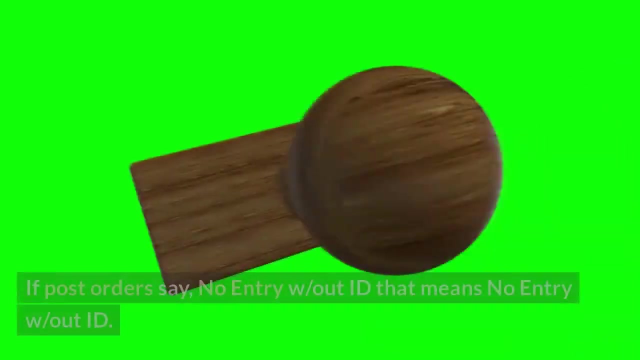 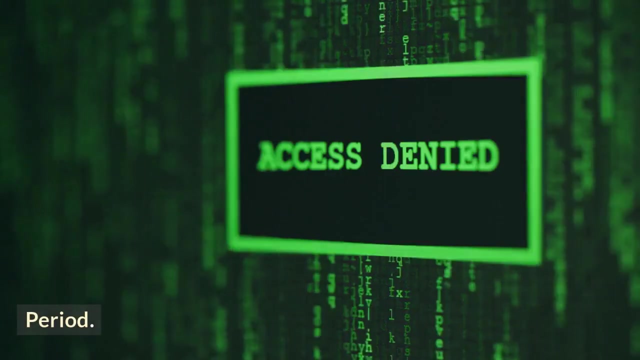 iris or retina scans. Also facial recognition software. From a security standpoint, facial recognition is the worst form of identification. Post-orders will have procedures for employees who forgot or lost their identification. If post-orders say no entry without ID, that means no entry without ID Period. Call a supervisor if any problem. 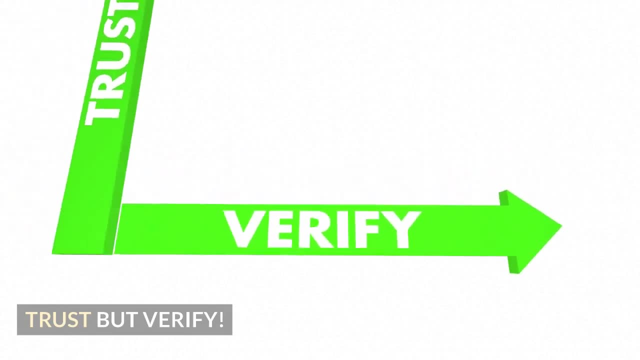 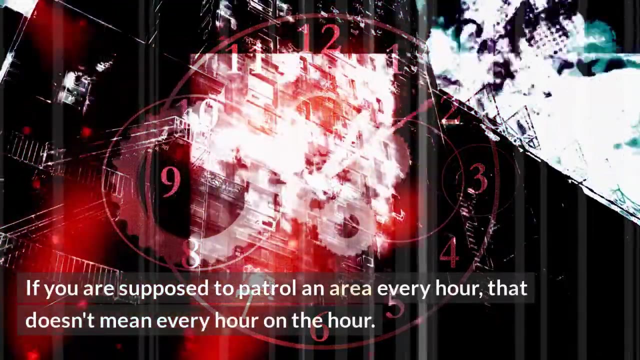 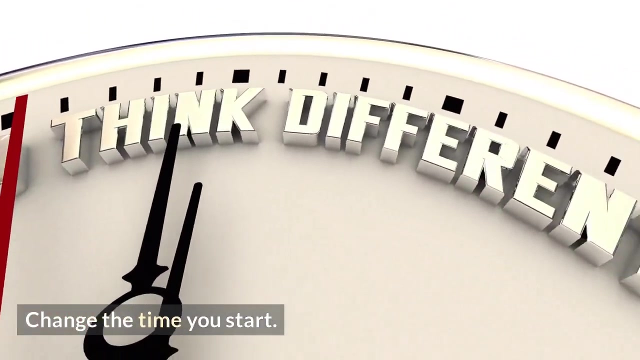 Trust but verify. Scatter your patrols. Don't be predictable. If you are supposed to patrol an area every hour, that doesn't mean every hour on the hour. Change the time you start: 5 minutes before or 5 minutes after. Change it up. 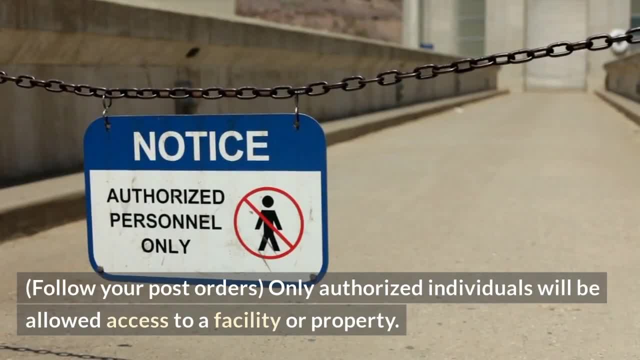 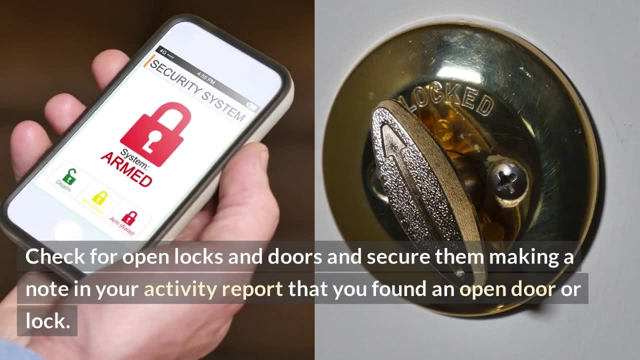 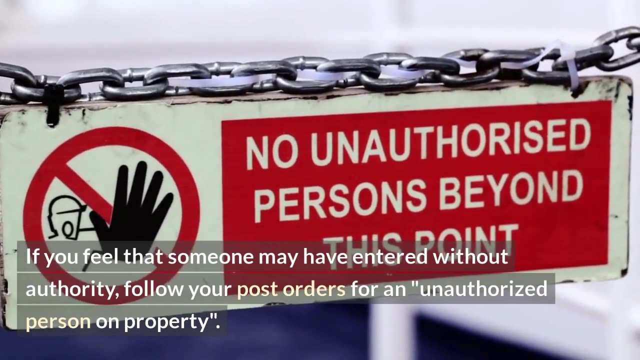 Follow your post orders. only authorized individuals will be allowed access to a facility or property. Check for open locks and doors and secure them, making a note in your activity report that you found an open door or lock If you feel that someone may have entered without authority, follow your post orders for an unauthorized person on property. 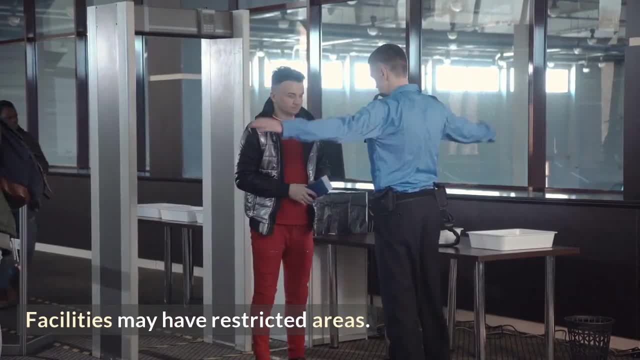 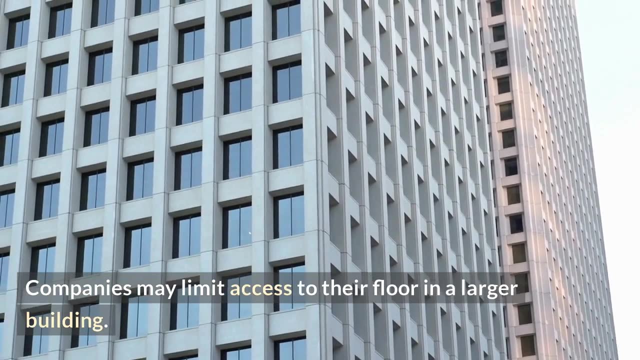 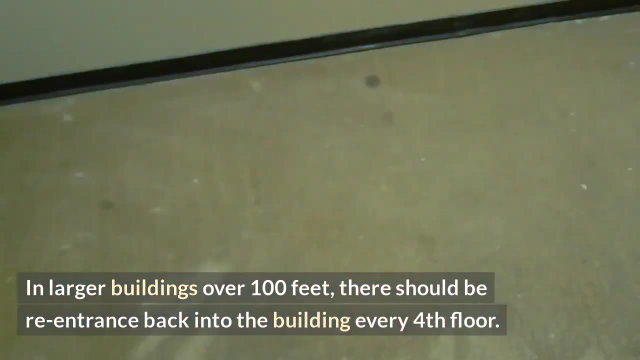 Facilities may have restricted areas. These areas are for authorized individuals. Companies may limit access to their floor in a larger building. In larger buildings over 100 feet there should be re-entrance back into the building. every fourth floor. They may have to follow check-in requirements or procedures.